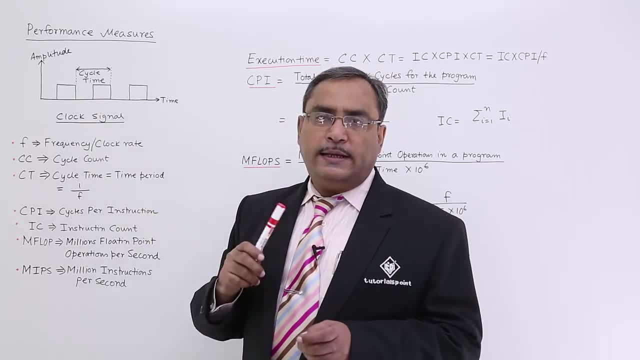 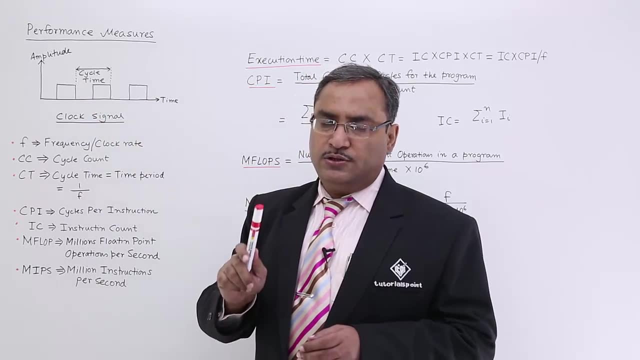 Or also can be called as cycle time or cycle period. So let us suppose, if you consider this point and this point, they are in the same phase. So that is why the difference between this time intervals will be known as the cycle time. 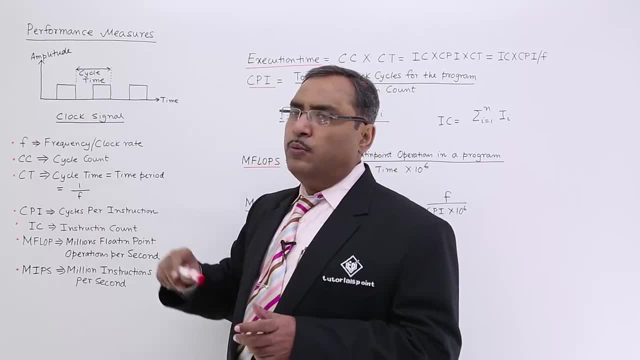 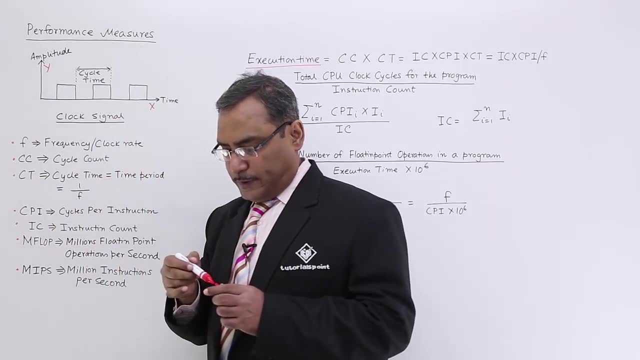 Because along the x-axis we are plotting time, Along the y-axis we are plotting the amplitude or the voltage. So let it be the x-axis and let it be the y-axis. So this is the clock signal. We have got the idea. 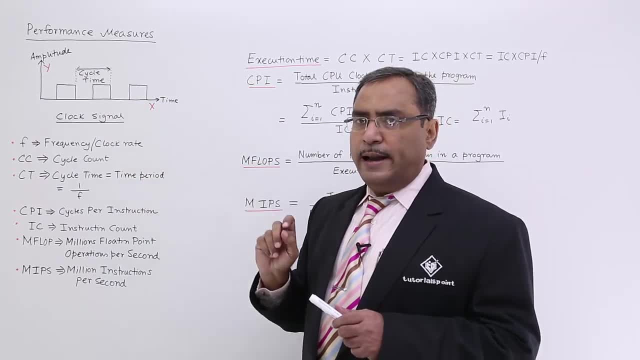 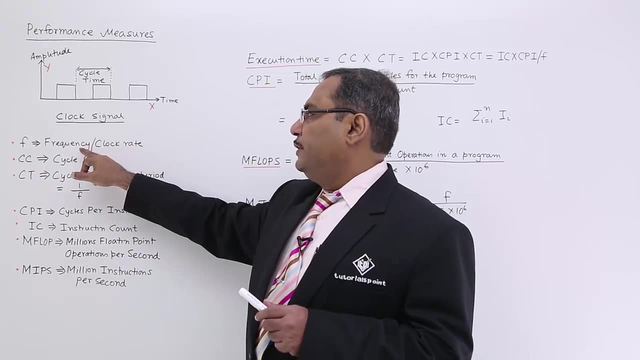 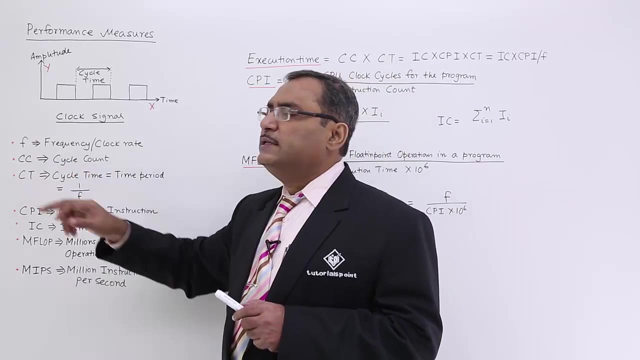 So what is the frequency? Frequency means number of time periods or clock cycles per second. So frequency means the clock rate. So frequency or clock rate can be denoted by F. This is my cycle count. Cc means cycle count. That means how many cycles are there within a particular time interval. So that is the cycle count. 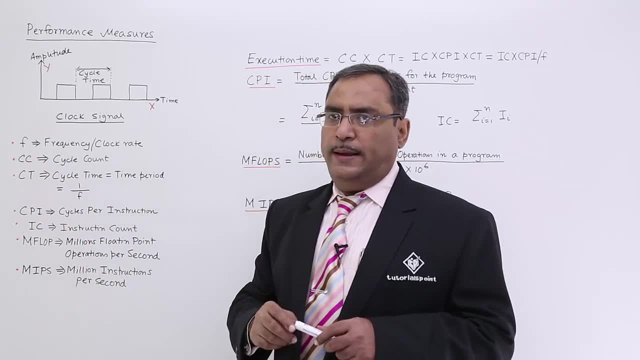 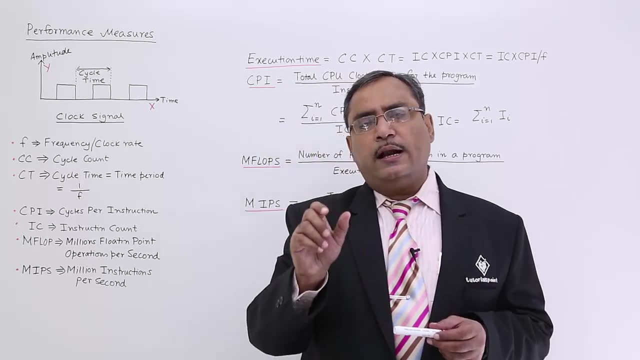 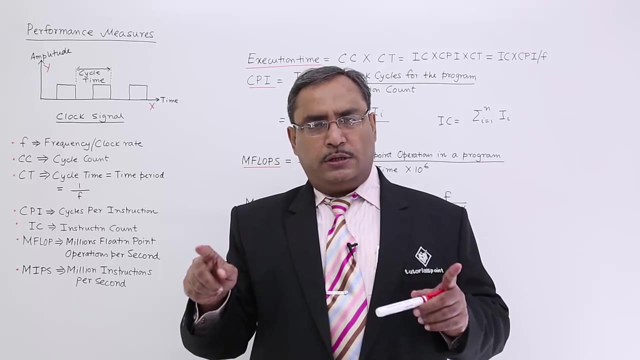 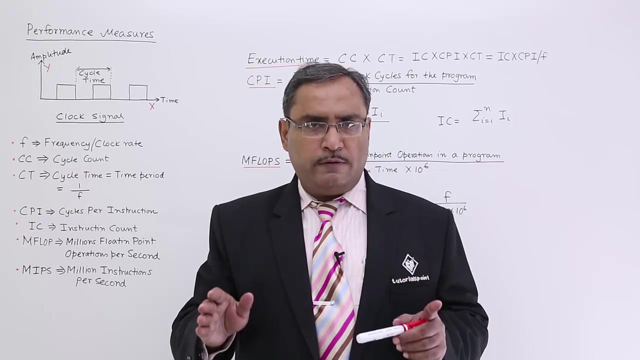 And we know that whenever a program executes a program is having minus multiple instructions. for executing each and every instruction i require a certain number of clock cycles. so when all instructions have got executed, then full instruction. all these instructions will have a cycle count. that means the total number of clock pulses required. 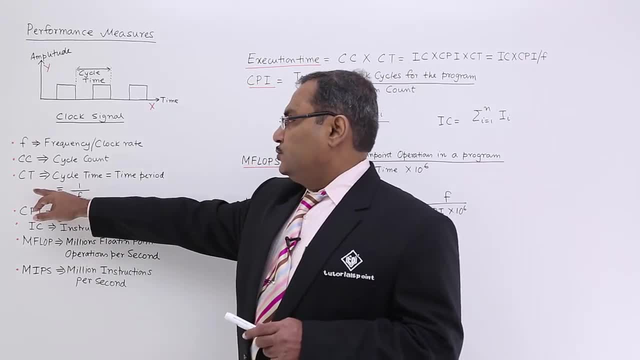 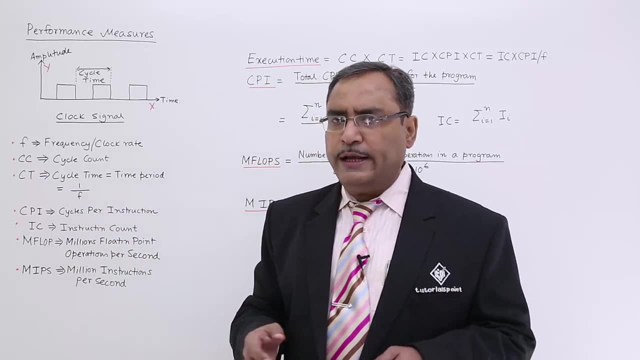 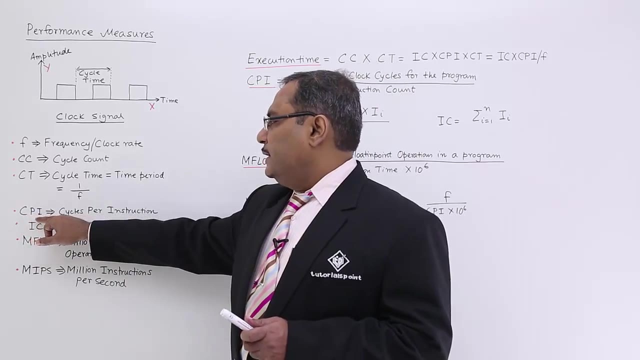 for the execution of the program. so cycle time means is equal to c, t or can be called as time period is equal to one by f. this is a very common formula, that is, ah, reciprocal of the frequency, will give you the time period cycles per instruction, c, p, i. so it is known. 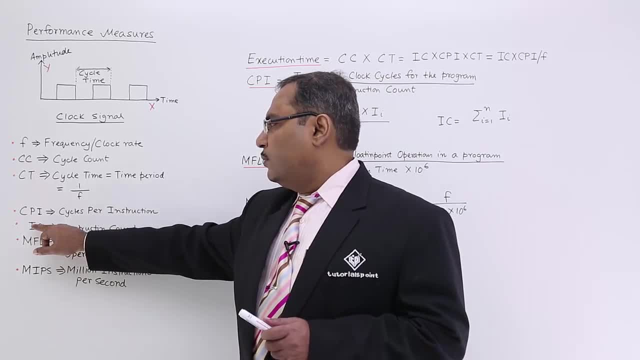 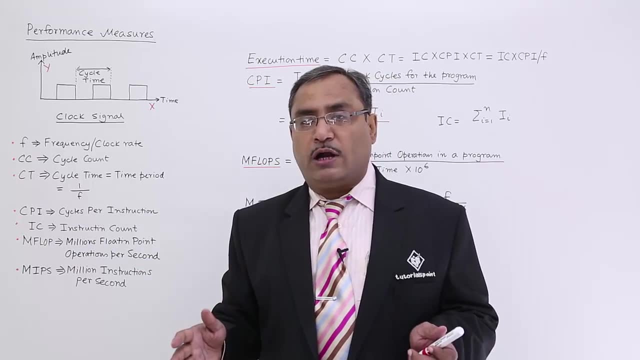 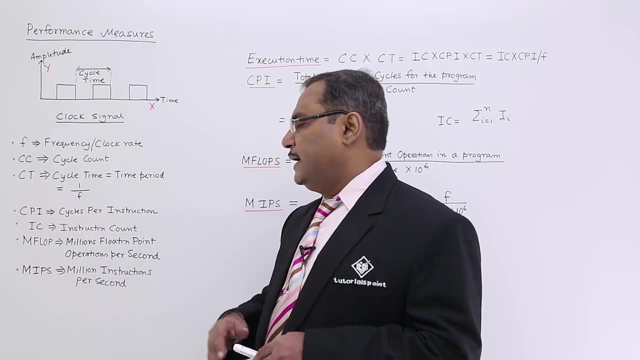 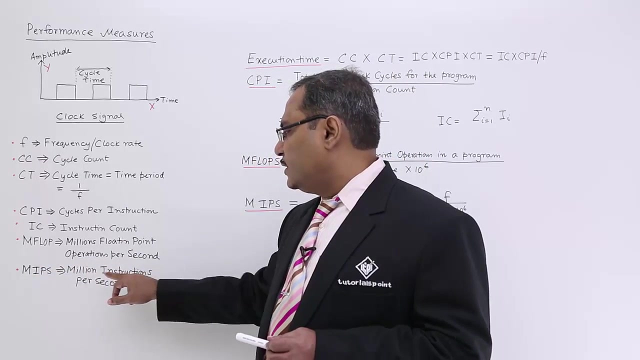 as cycles per instruction. this is i c. what is c p i? i have discussed that one later. so what is i c? instruction count means what means number of instructions? m prop. m prop means million floating point operations per second. m prop, also called as m props. and last one is a m i p? s, that is, million instructions per second. 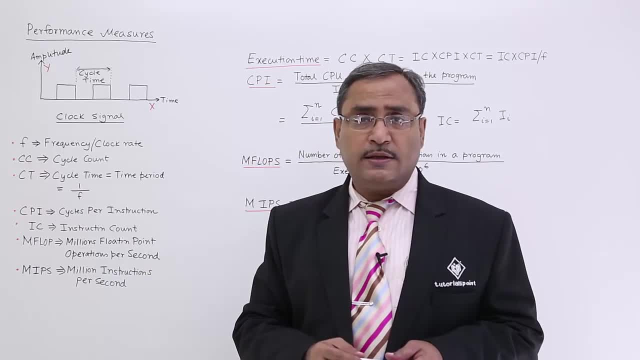 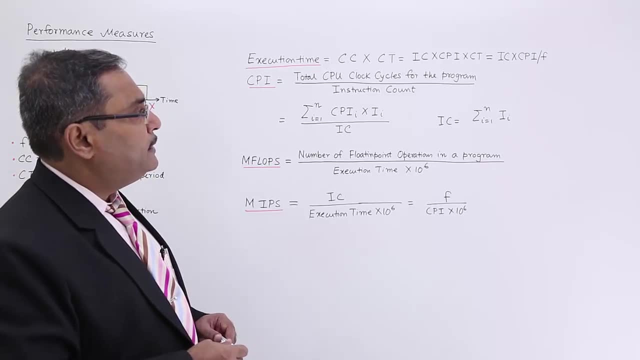 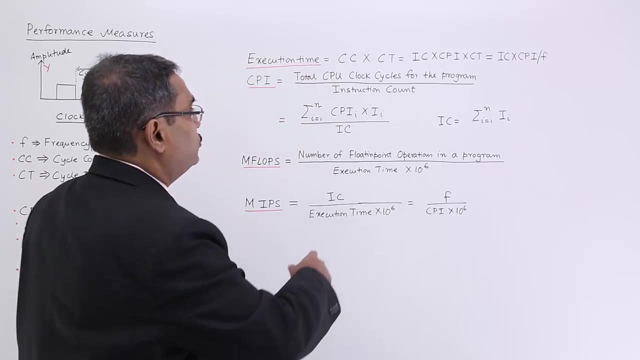 so m, prop, m, i, p, s, these are the performance measures of a system. so let us go for the detailing of the of this formula now. execution time means cycle count into that is a cycle duration, cycle timing. good, so we are having the c, c and respective c t, so it is also mentioned. 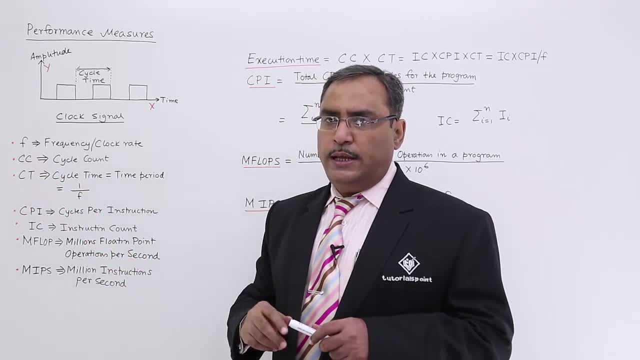 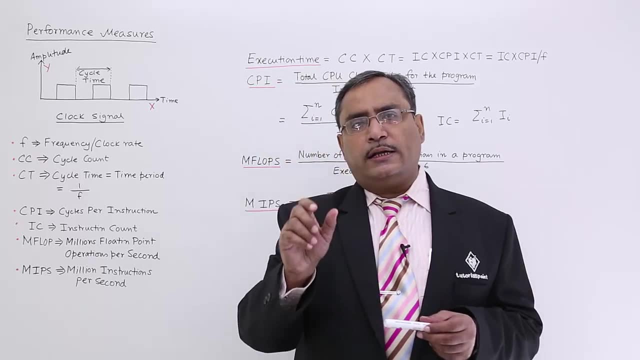 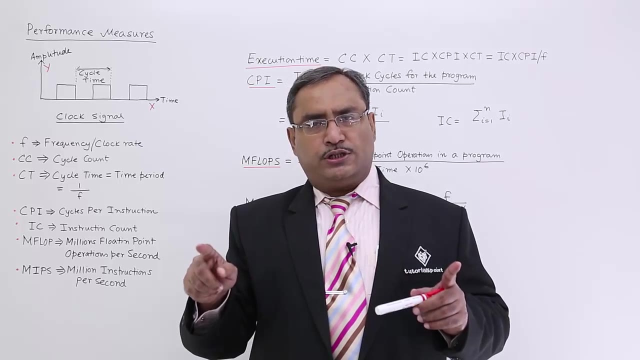 And we know that whenever a program executes, a program is having minus. So we have multiple instructions. For executing each and every instruction I require a certain number of clock cycles. So when all instructions have got executed, then full instruction. all these instructions will have a cycle count. 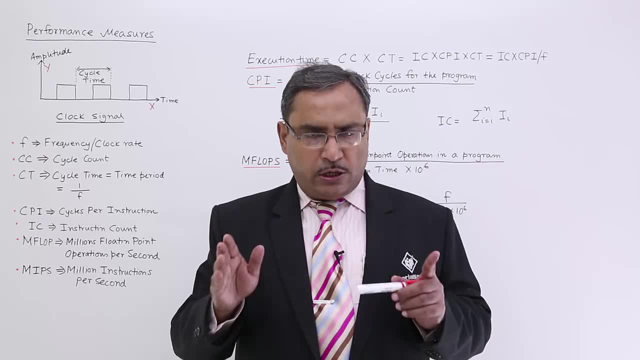 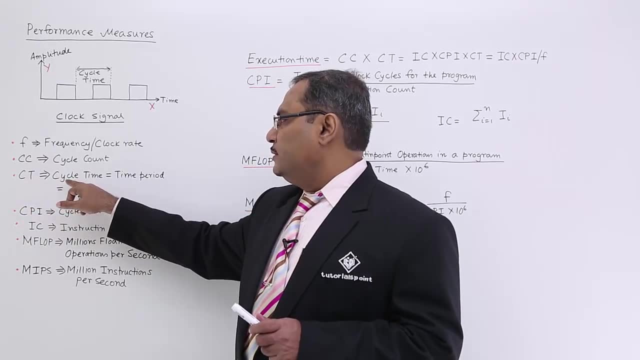 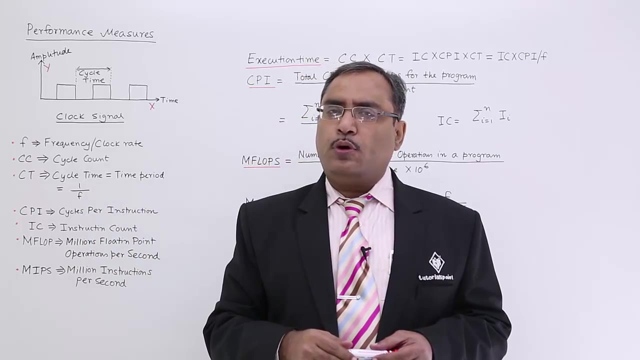 That means the total number of clock pulses required for the execution of the program. So cycle time is equal to CT, or can be called as. time period is equal to 1 by f. Okay, So this is a very common formula that is reciprocal of the frequency will give you the time period. 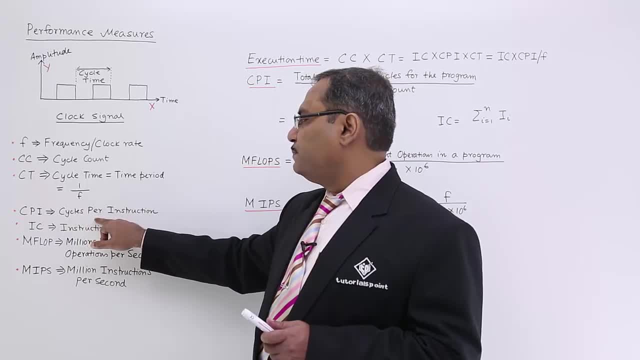 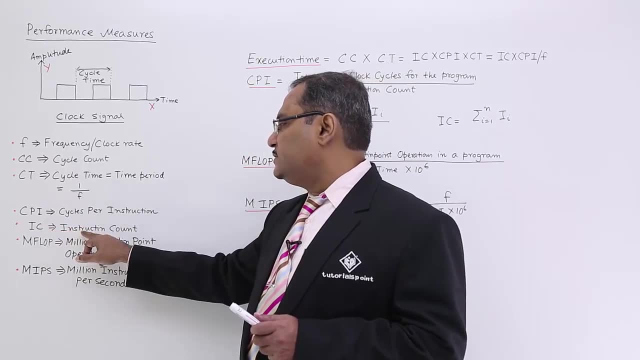 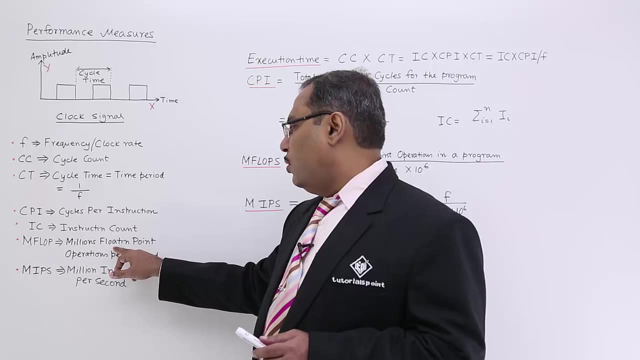 Cycles per instruction, CPI, So it is known as cycles per instruction. This is IC. What is CPI? I have discussed that one later. So what is IC? Instruction count Means what Means number of instructions, MPHROP. MPHROP means million floating point operations per second. MPHROP, Also called as MPHROPs. 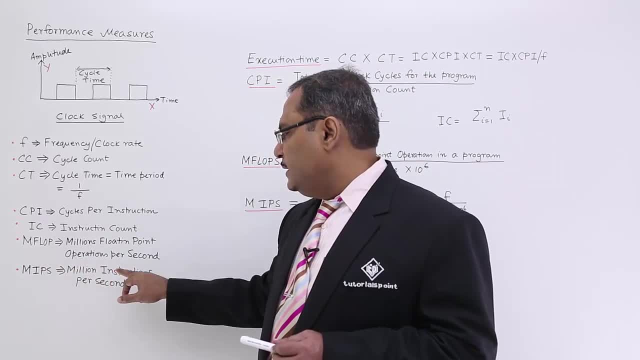 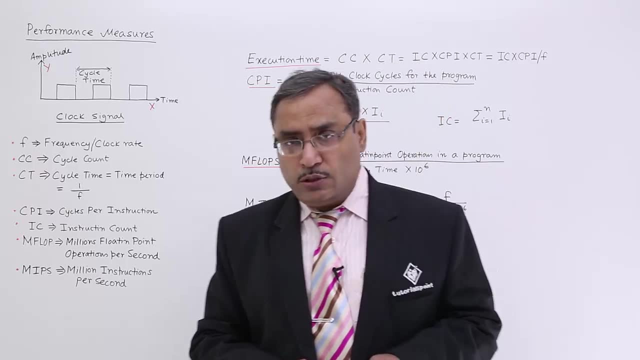 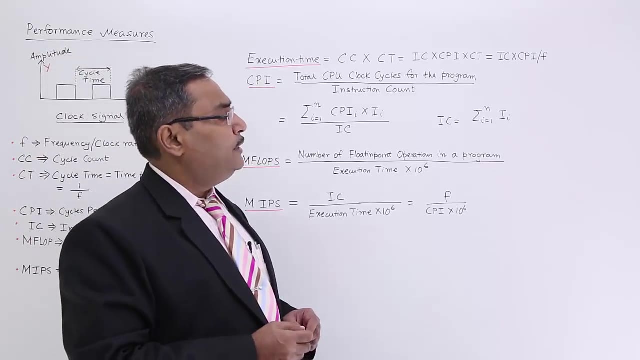 And last one is a MIPS. That is million instructions per second. So MPHROP, MIPS, these are the performance measures of a system. So let us go for the detailing of this formula Now. execution time means cycle count into that is a cycle duration, cycle timing- Good. 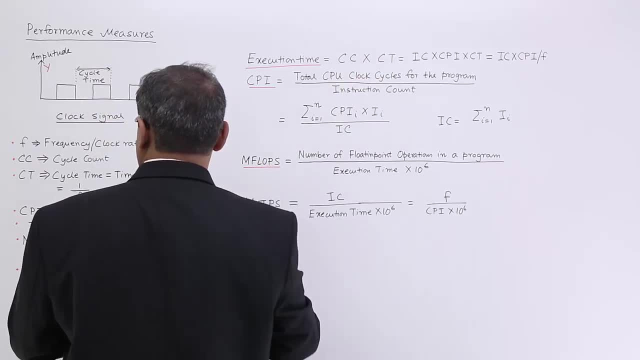 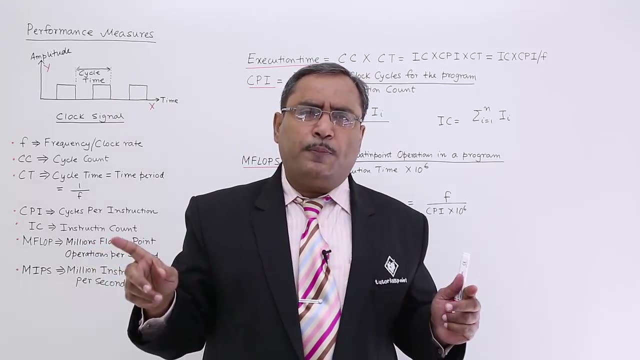 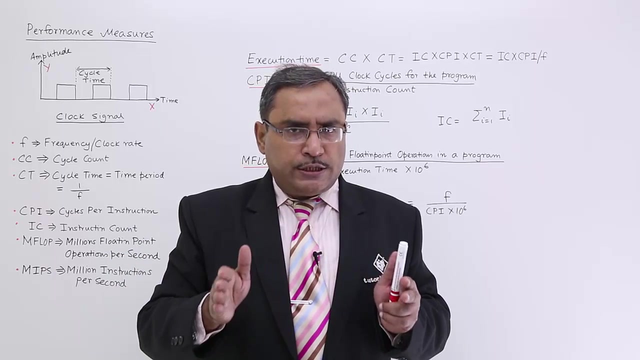 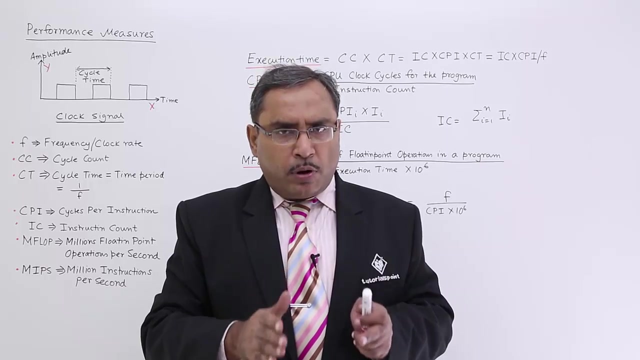 So we are having the CC and respective CT. So it is also mentioned that CC and CT. Okay, Now see. So CC means total number of clock cycles required for the execution of a program. A program is nothing but collection or mix of multiple instructions. Depending upon the instruction category, number of clock cycles required to execute that instruction may vary. 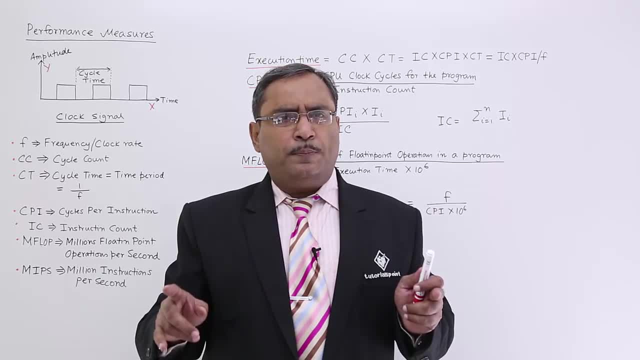 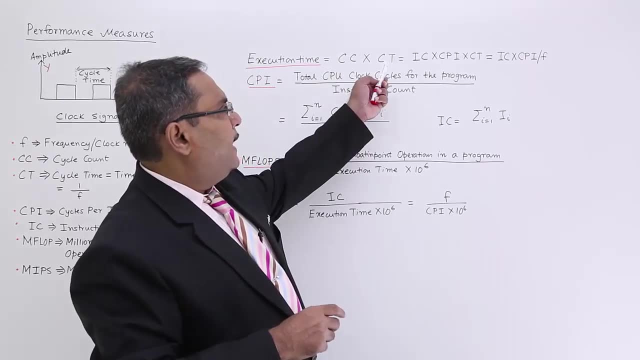 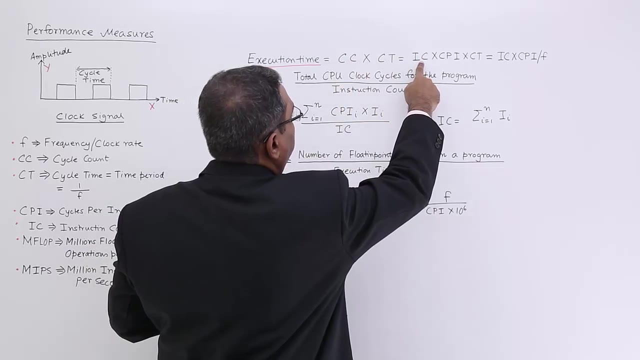 So in that case, so total number of clock cycles required- that is known as a cycle time Cycle count- will be multiplied with this particular cycle time and that will give you the total execution time of the program. So this cycle time can be calculated in this way. That is the instruction count into CPI, That is the cycles per instruction. 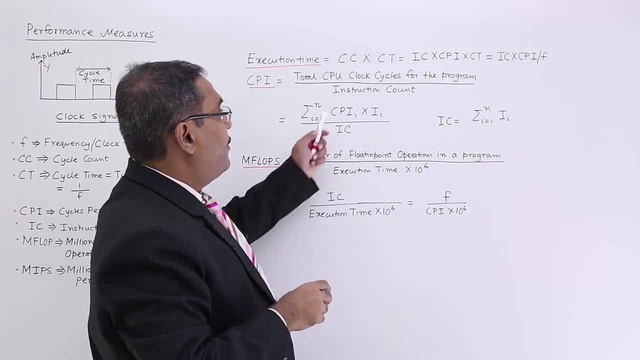 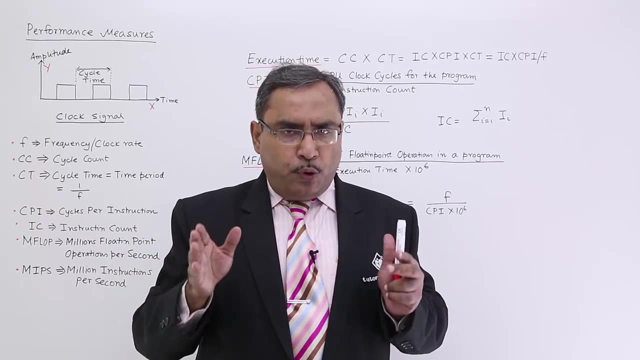 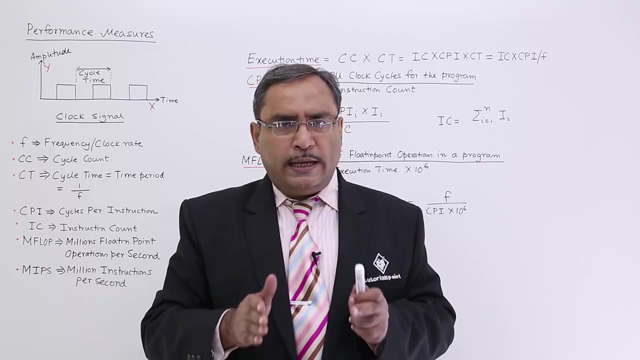 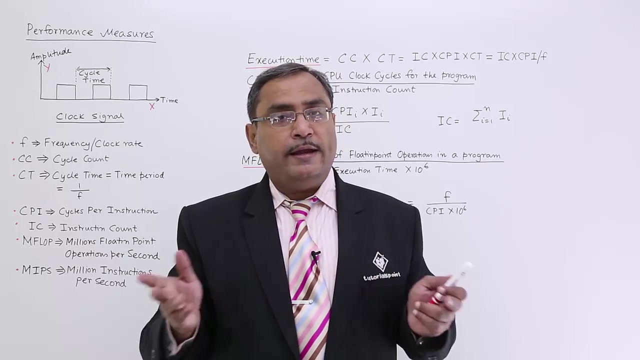 that c, c and c? t. ok, now see. so c? c means total number of clock cycles required for the execution of a program. a program is nothing but collection or mix of multiple instructions. depending upon the instruction category, number of clock cycles required to execute that instruction may vary. so in that case, so total number of clock. 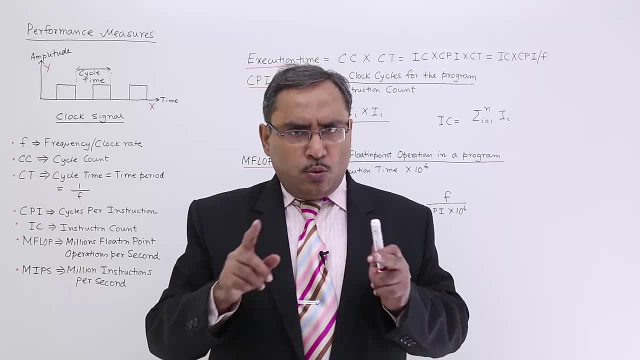 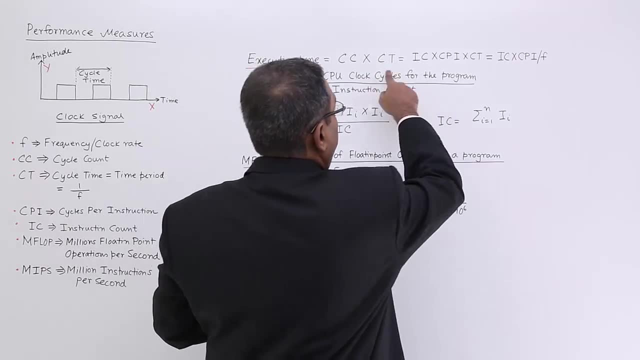 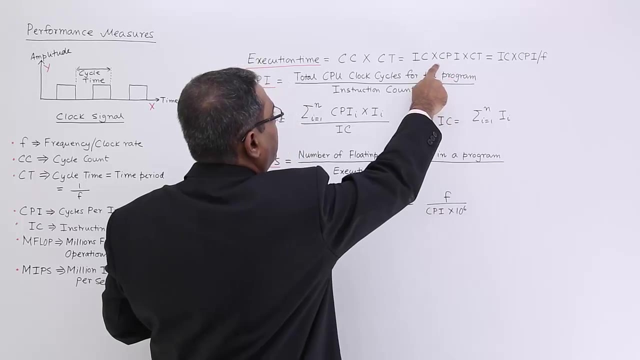 cycles required. that is known as a cycle time. cycle count will be multiplied with this particular cycle time and that will give you the total execution time of the program. so this cycle time can be calculated in this way. that is the instruction count into into c, p, i, that is the cycles per instruction. so instruction count into cycle per instruction. 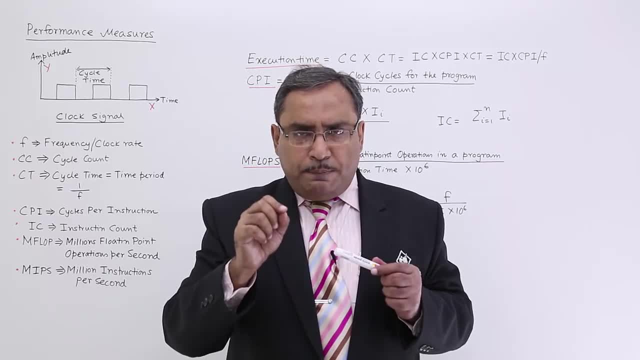 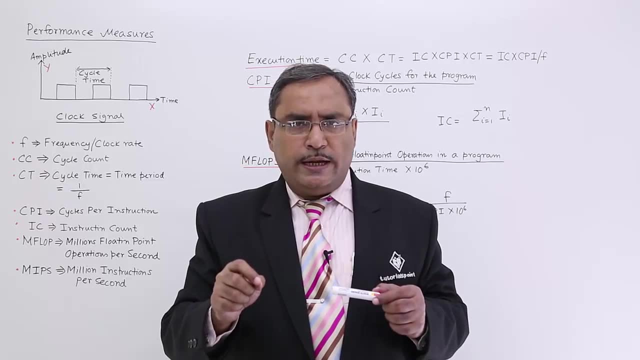 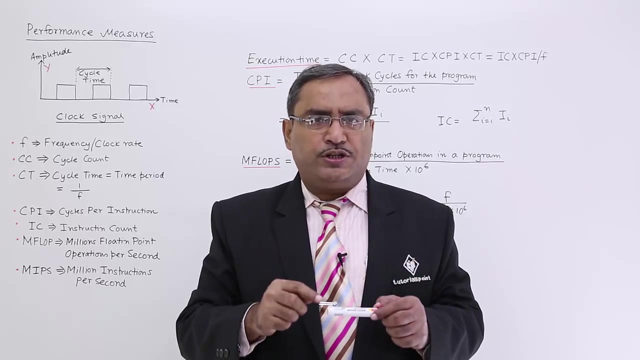 that means as each and every instruction, depending upon its category, whether it is load or store instruction, whether it is a branching instruction, whether it is an a? l? u instruction. so depending upon the instruction type, the cycles per instruction may vary. so if you go for the average of cycles, 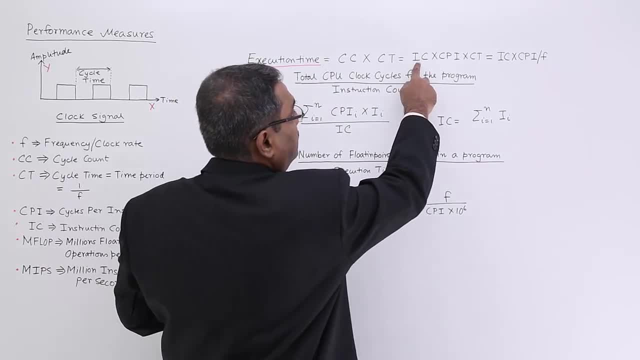 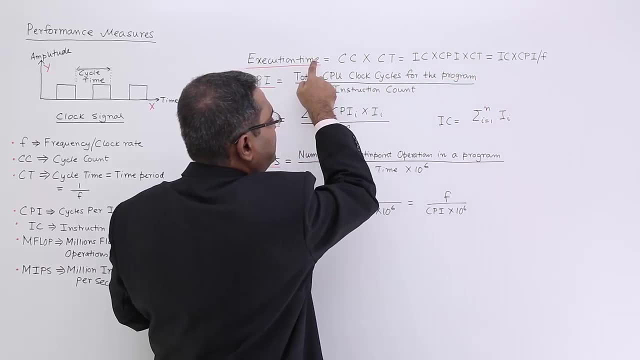 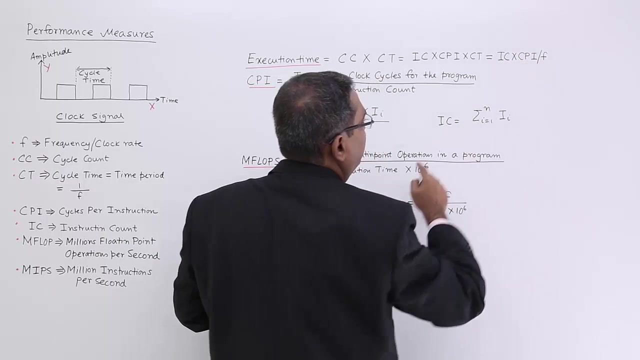 per instruction required and that is known as a c p i. so instruction count into c p i, into cycle duration. cycle time will give you the corresponding execution time of a program and this c? t can be by 1, by F. So IC into CPI, by F will be the cycle, will be the execution time. Now let me discuss. 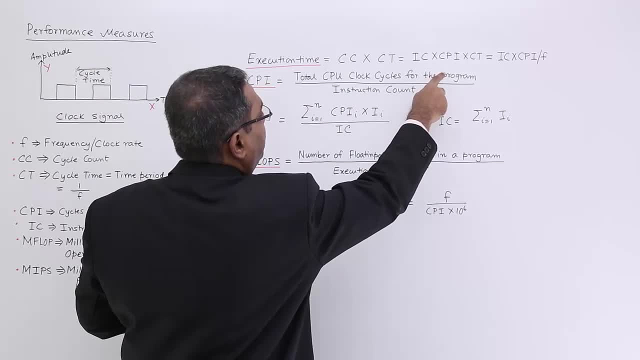 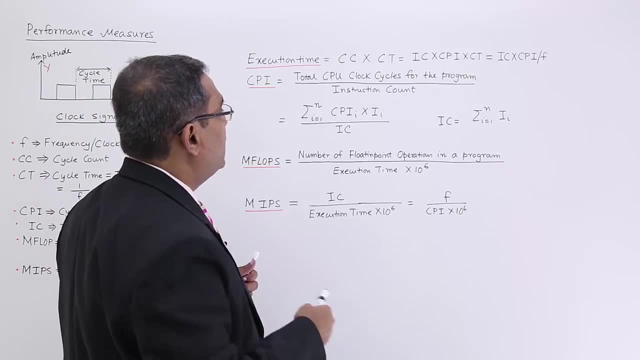 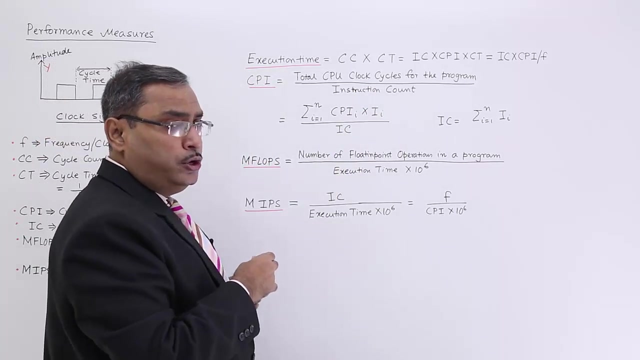 this CPI, Total CPU clock cycles for the program required by the instruction count will give you this particular measure of this particular CPI. So instruction count will give you the idea of the CPI. I told you that, depending upon the category of the instructions, number of clock. 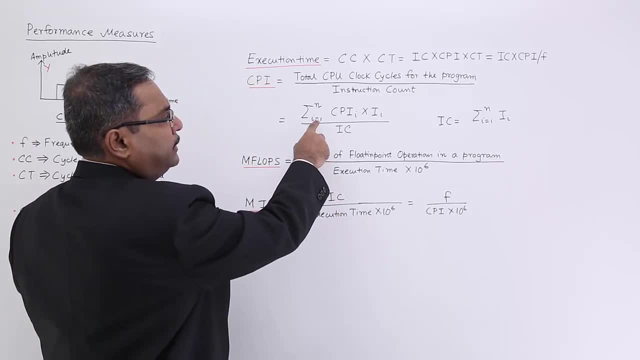 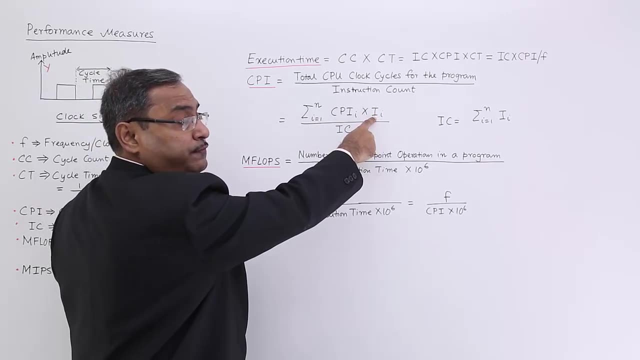 cycles required to execute that instruction may vary. So that is why let us suppose we are having n categories. So n categories i is the number of instructions for that very particular category and this is the CPI, that is, the cycles per instruction required for that very particular. 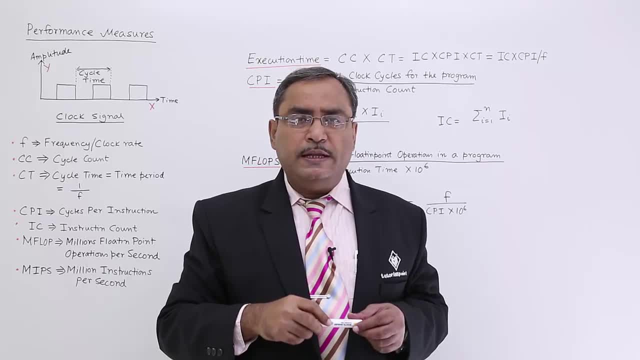 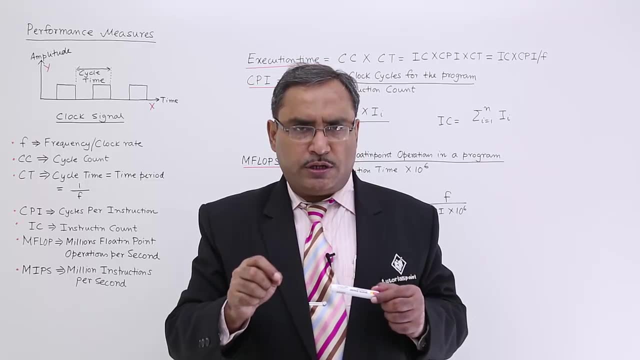 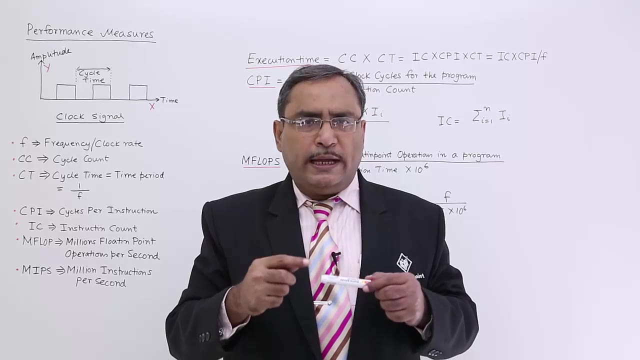 So instruction count into cycle per instruction. That means, as each and every instruction, depending upon its category, whether it is load or store instruction, whether it is a branching instruction, Whether it is an ALU instruction, So depending upon the instruction type, the cycles per instruction may vary. 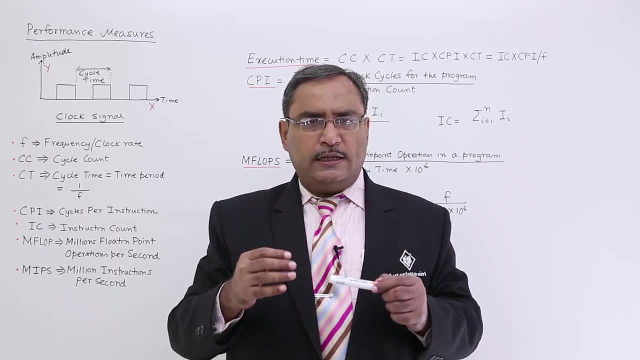 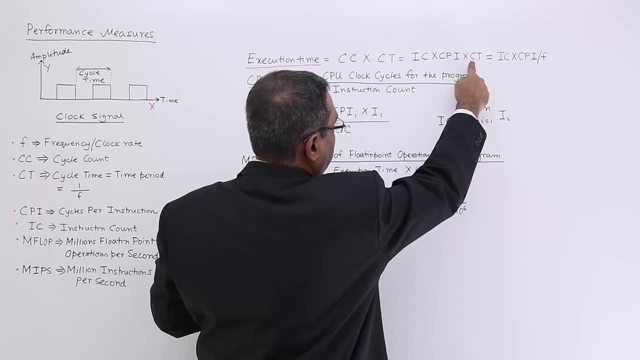 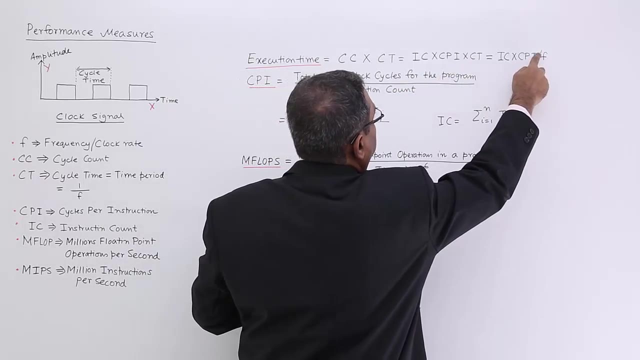 So if you go for the average of cycles per instruction required and that is known as a CPI, So instruction count into CPI, into cycle duration. cycle time will give you the corresponding execution time of a program and this CT can be written by 1, by F. 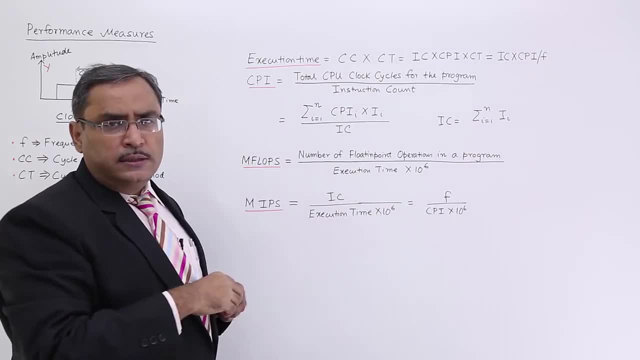 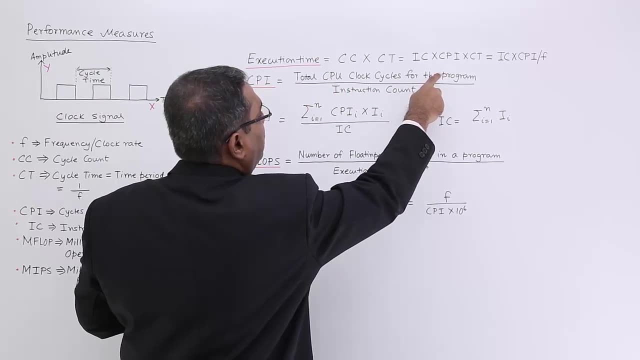 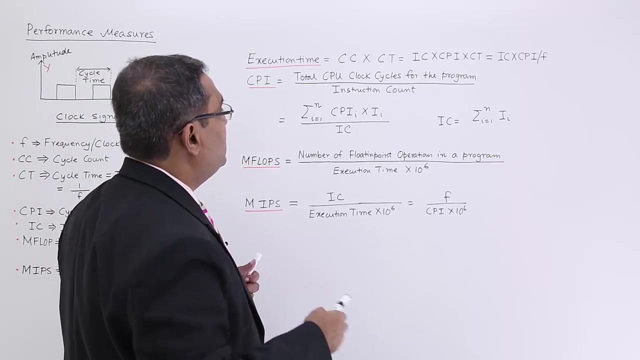 So IC into CPI, So IC into CPI by F will be the cycle or will be the execution time. Now let me discuss this CPI. Total CPU clock cycles for the program required by the instruction count will give you this particular measure of this particular CPI. 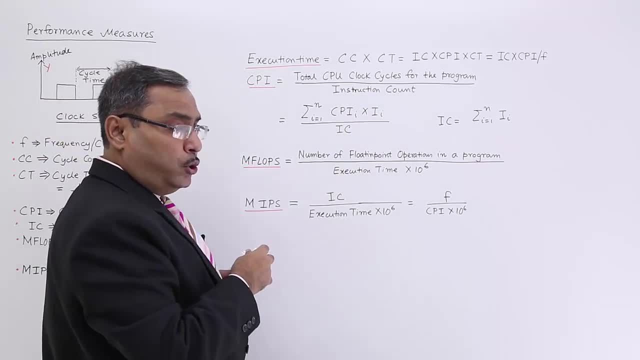 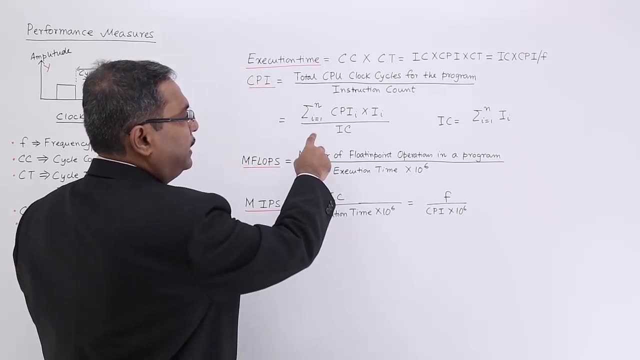 So instruction count will give you the idea of this CPI. I told you that depending upon the category of the instructions, number of clock cycles required to execute that instruction may vary. So that is why, let us suppose we are having N categories. 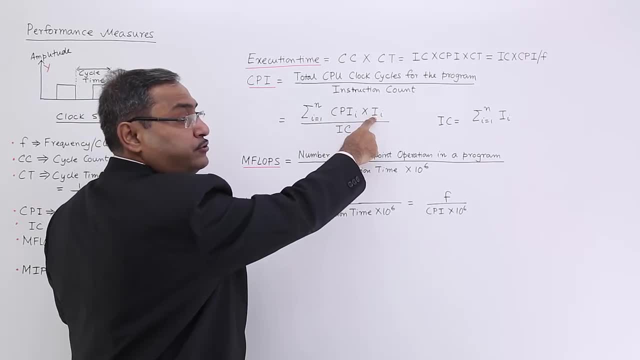 So N categories I is the number of instructions for that very particular category and this is CPI. That is the cycles per instruction required for that very particular category. So if you go on multiplying them I am getting the total CPU clock cycles for the program. 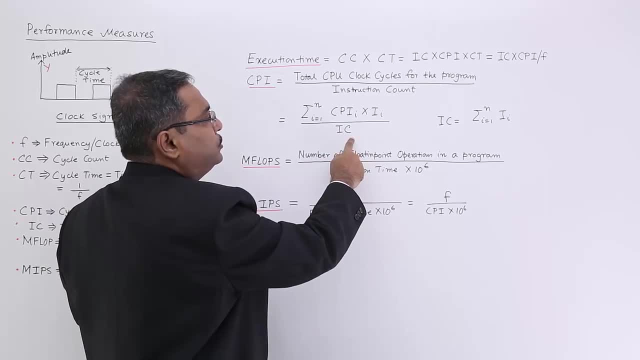 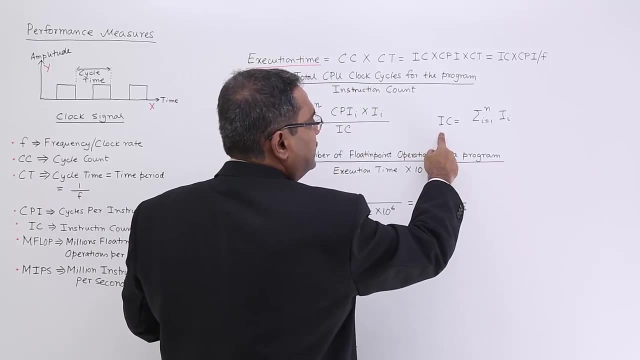 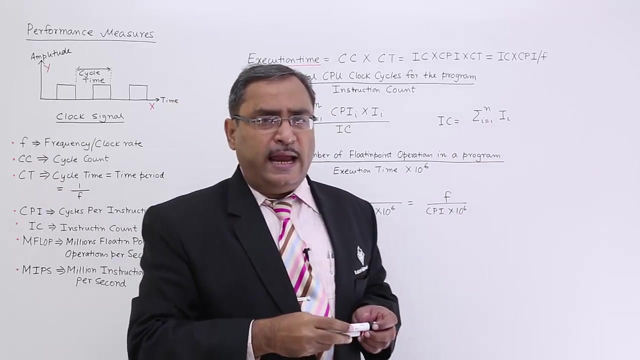 And then I am dividing it with this instruction count. So I am getting this CPI. So that is the average clock cycles. This is the maximum clock cycles for the general instruction, And this IC is nothing but sigma. That is the summation of II, where I is ranging from 1 to N. 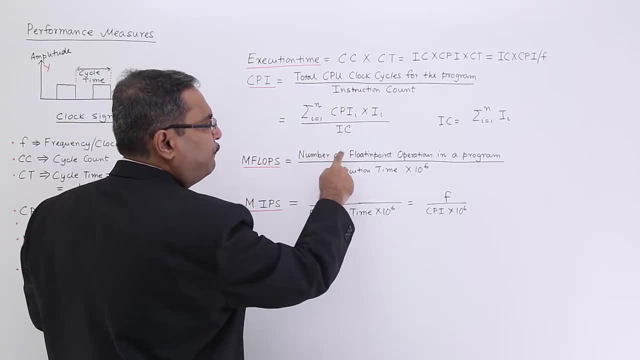 What is N? N is the number of categories, Now M props, So number of floating-point operations in a program by execution time, So that you are getting the M props. Why it 10 to the power of 6 is there. 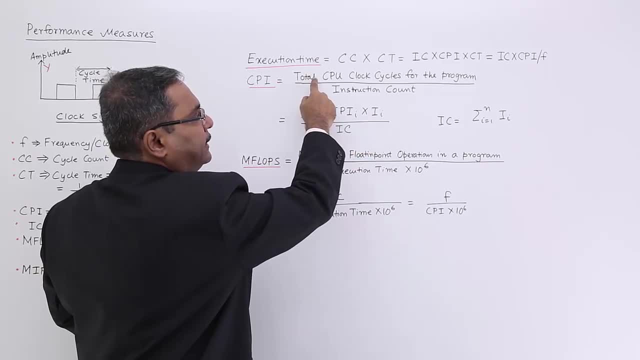 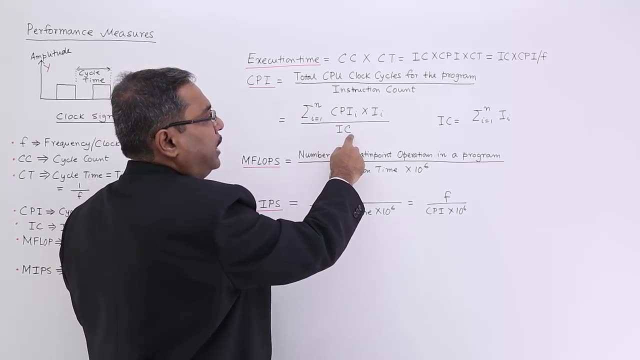 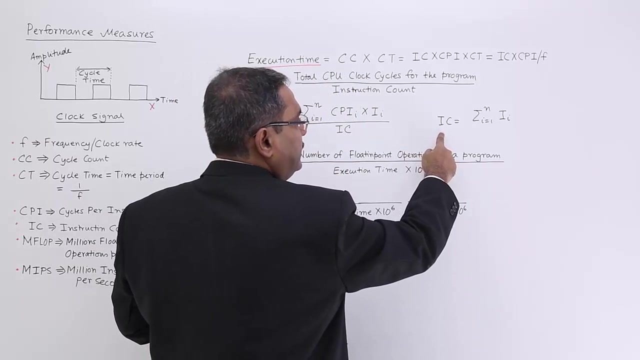 category. So if you go on multiplying them I am getting the total CPU clock cycles for the program, and then I am dividing it with this instruction count, So I am getting this CPI. So that is the average clock cycles per instruction, and this IC is nothing but sigma. That is the summation of 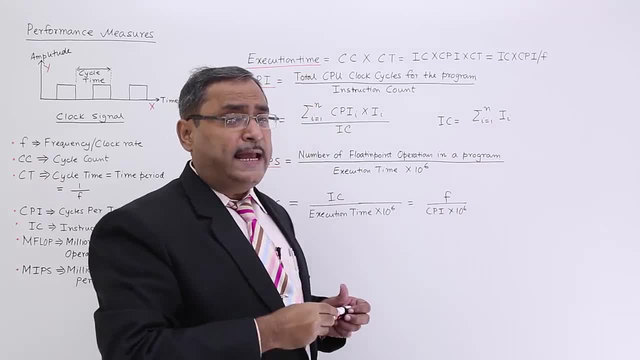 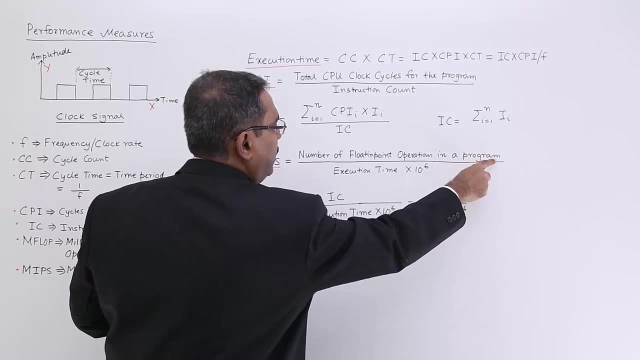 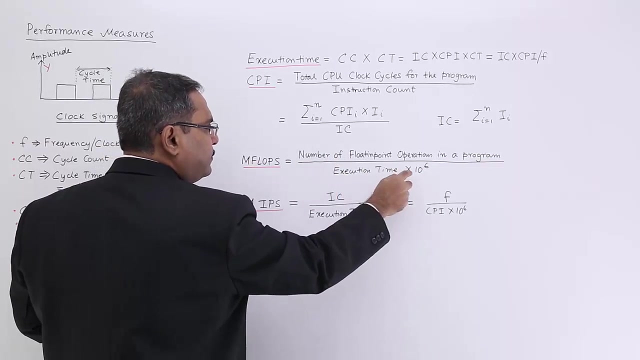 ii, where i is ranging from 1 to n. What is n? n is the number of categories, Now m props, So number of floating point operations in a program by execution time, So that you are getting, you are getting the m props. Why 10 to the power of 6 is there, Because I am going for million. So 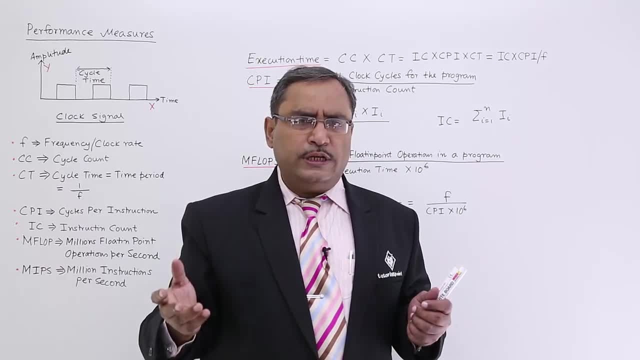 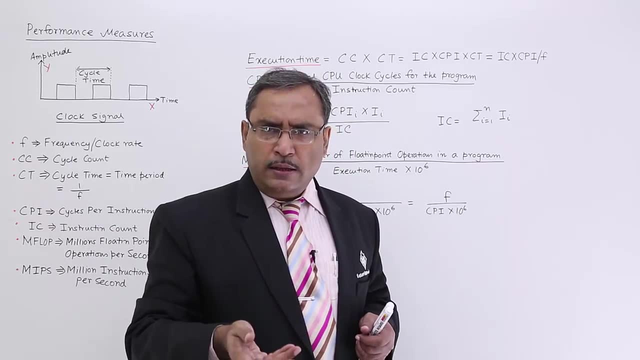 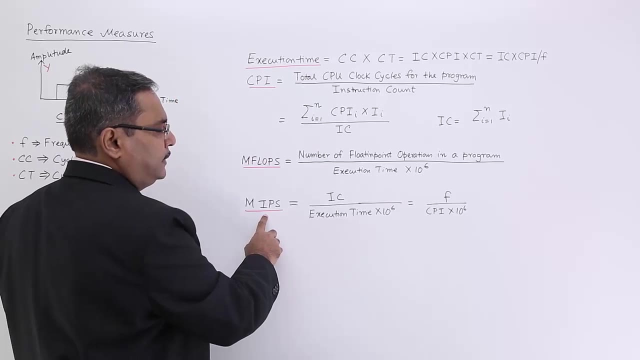 this particular value will be a huge value. So it is better to take the value with the scale of million. So that is why you know, million means mega. million means mega. mega means 10 to the power of 6.. So by 10 to the power of 6.. MIPS it is IC. that is the total instruction, count by 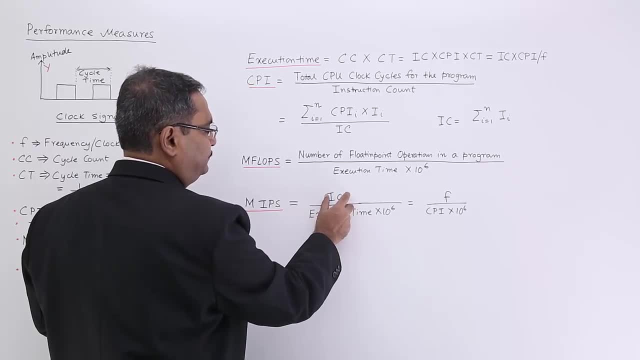 execution time: MIPS. total instruction count by the execution time will be the MIPS, but it is m is there? million is there. So it is a total instruction count by the execution time, So by 10 to the power of 6.. Million means mega, means 10 to the power of 6.. So that is the formula for. 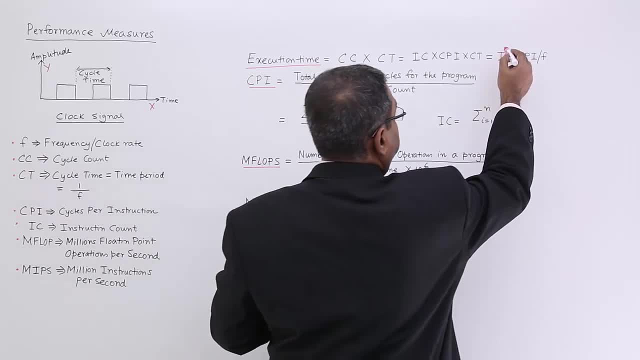 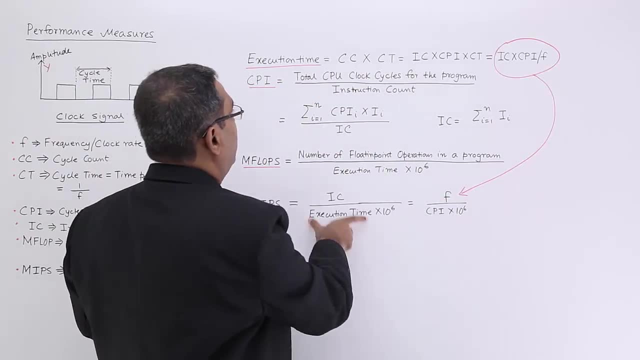 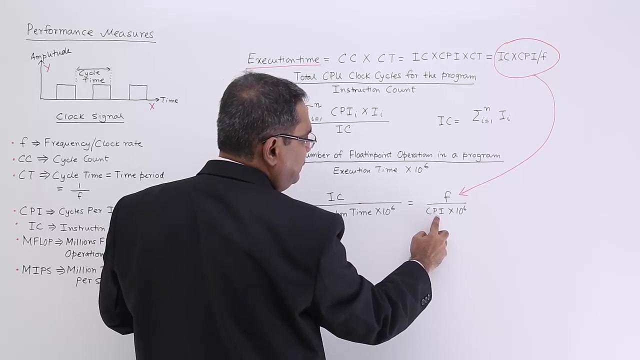 MIPS. So now I have used this particular formula. I have used it here. Just see what is execution time. Execution time is equal to IC into CPI by F. So execution time is equal to IC into CPI by F and IC. IC will cancel out each other, So I will be. I shall be remaining with. 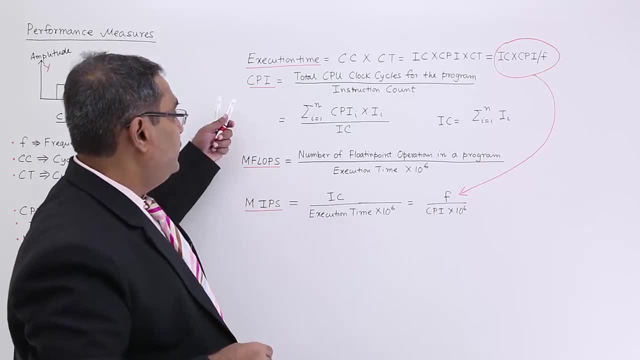 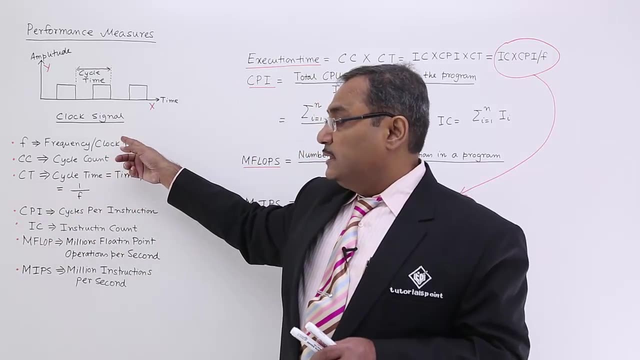 F by CPI into 10, to the power of 6.. So in this way, MPROPS, MIPS, CPI. I have done the calculation, along with the execution time and so on. So this is these are the abbreviations. This is the clock. 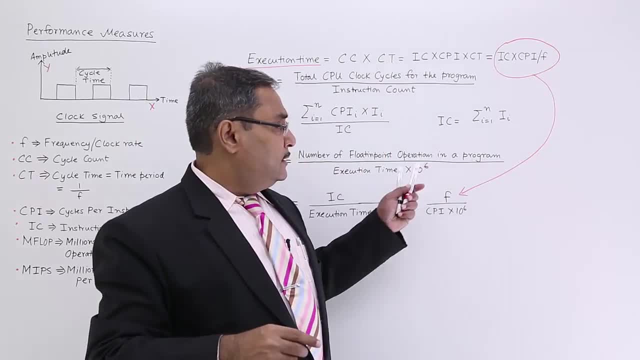 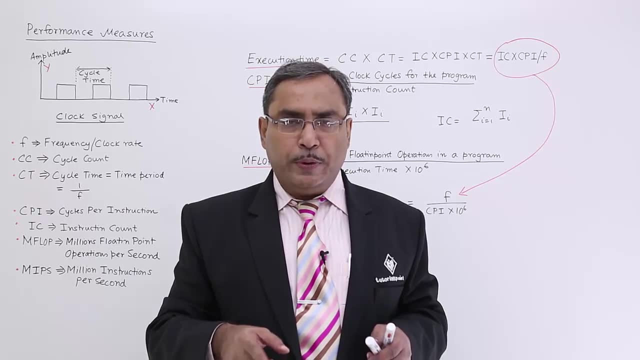 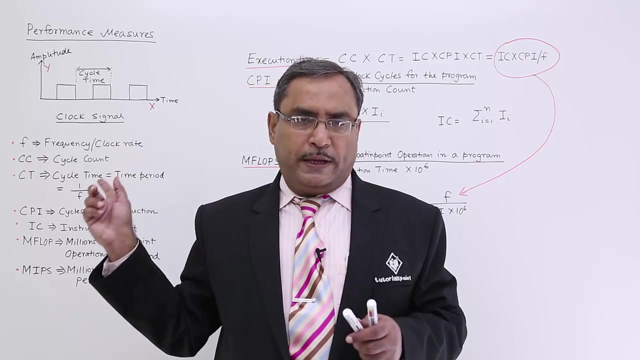 diagram, clock signal diagram or timing diagram. This is the respective formulas I will be equating. So please watch my next video where we shall solve one numerical problem: probable gate question. numerable numerical problem on this particulars Topic. considering all these aspects, on these performance measures. 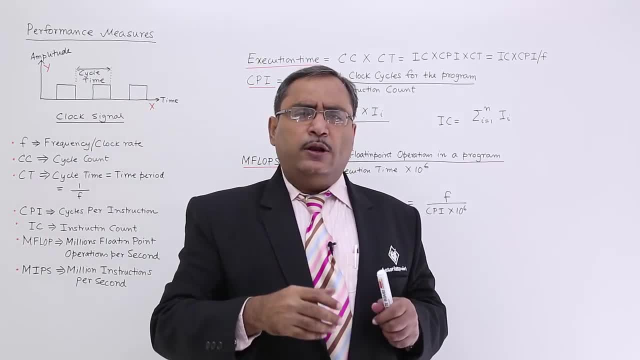 Because I am going for million. So we know that is This particular value will be minus, So that is not happening- be a huge value. So it is better to take the value with the scale of million So that